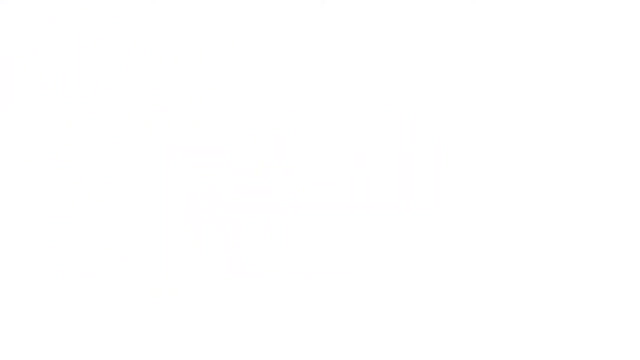 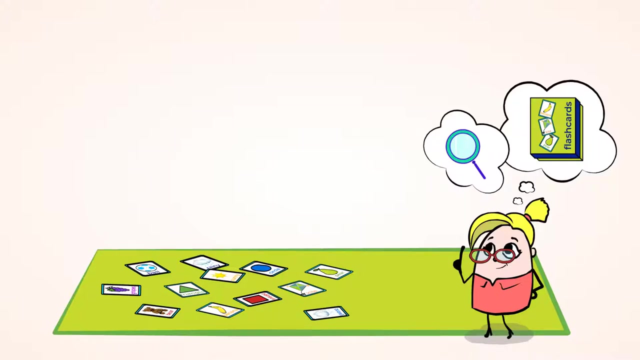 Hello, this is Mighty Owl. Oh no, Jenny's flashcards fell out of their box. They are spread out all over the floor. Jenny wants to put them back in the box in a way she can find them easily when she looks for them next. 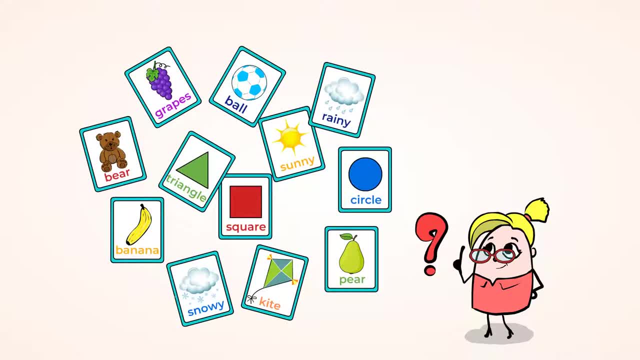 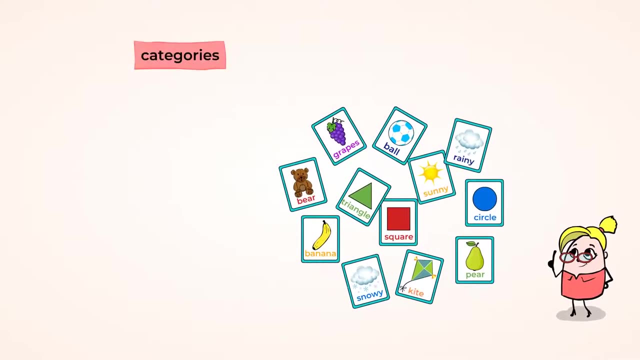 Let's give her a hand. What pictures do you see on the flashcards? I see a banana, a circle, a teddy bear, a rainy day, But these cards don't really seem like they go together. Let's help Jenny organize them into categories. 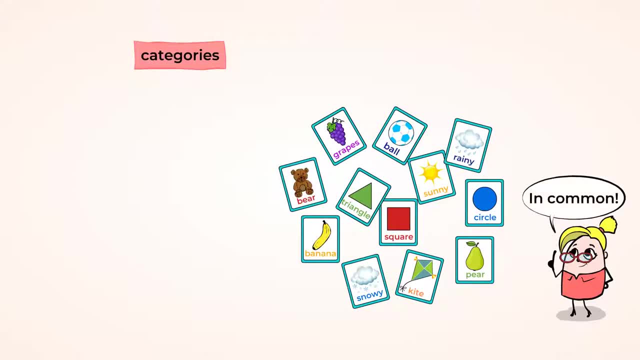 A category is a group of things that all have something in common. Well, we have the banana card, which we know is a fruit. so I suggest we make a fruit category. We can put the banana card in the fruit category by just moving it over to make its own pile. 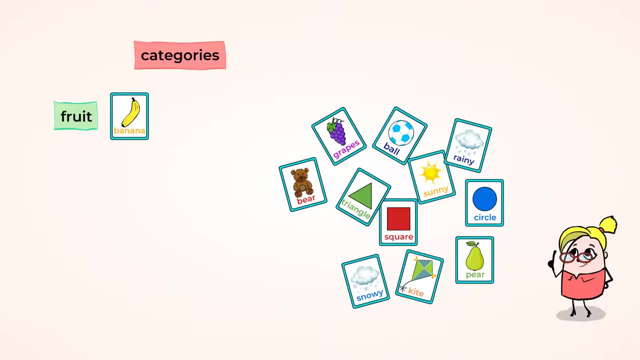 What other cards could go in the fruit category? Hmm, grapes are a fruit. Let's move that card next to the banana. What else? Aha, a pear is a fruit too. The fruit category has a banana, grapes and a pear. 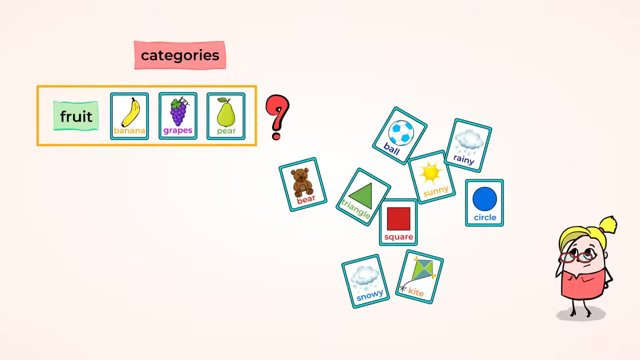 What do they all have in common? Well, they're all fruits. Well done, completing the first category. Jenny's cards are starting to look more organized already. Okay, let's make another category now, The shape category. We can start with the circle, because a circle is a shape. 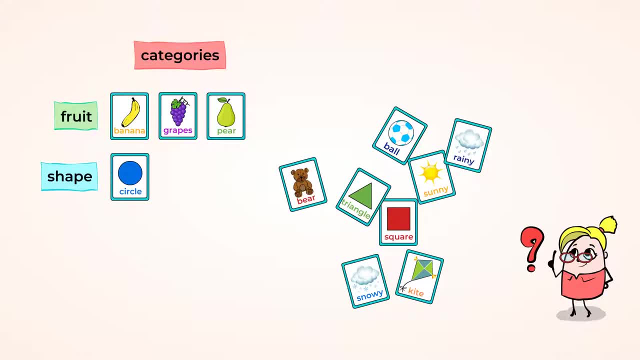 What other shapes do you see? Let's see, let's see. Oh, a triangle is a shape. We can put it in the shape category too. Anything else, A square, is a shape. So what do all of these cards have in common? 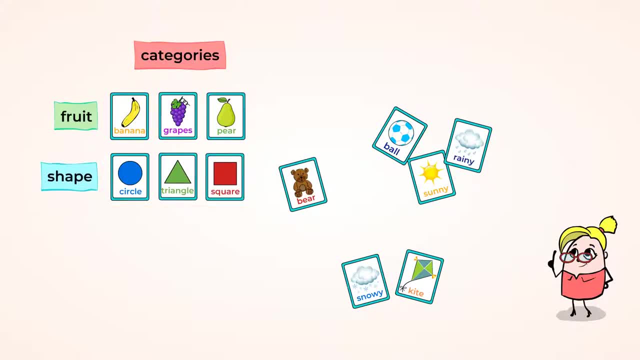 Right, they're all shapes, Nice work. Next up, The toy category. Ooh, my favorite. Which of these cards have toys on them? This one has a teddy bear, which is definitely a toy. A soccer ball is also a toy, so let's move it to the toy category too. 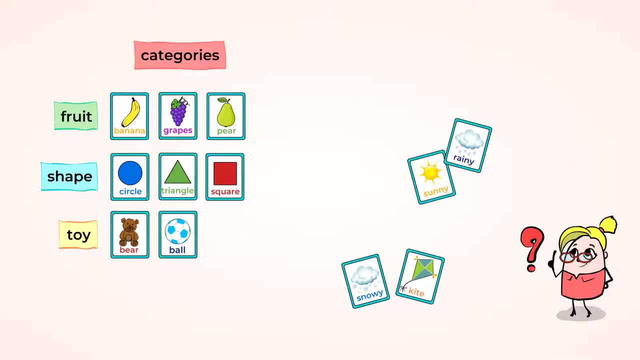 Do you see another toy? You got it. The kite is a toy. The teddy bear, soccer ball and kite are all toys. You're doing a great job sorting Jenny's cards. It looks like we're almost done. There's one category left. 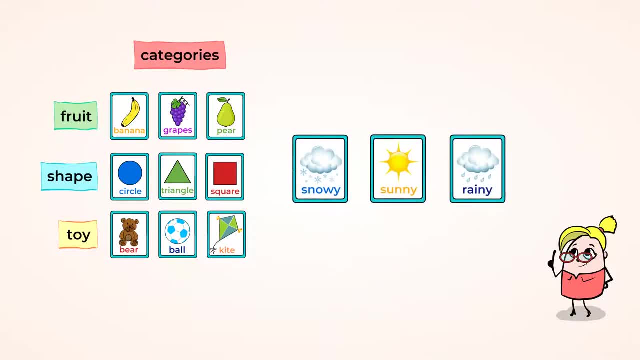 Let's look at the cards to figure out what their category is. I see a rainy day, a sunny day and a snowy day. What do they all have in common? Hmm, Those are all pictures we use to talk about the weather. 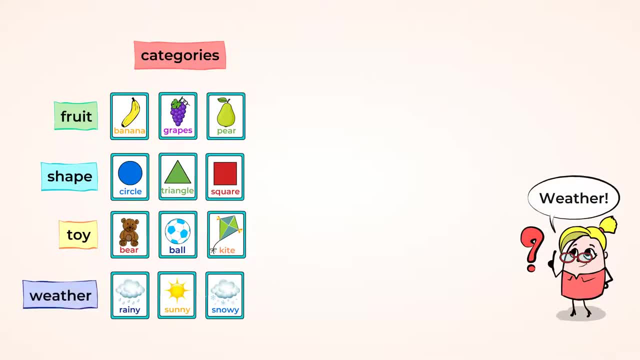 So the last category is weather. Woohoo, We sorted all of Jenny's cards into four categories: Fruits, shapes, toys and the weather. When you are sorting, you can make as many categories as you want. You can make four, just like we did, or two or three categories. 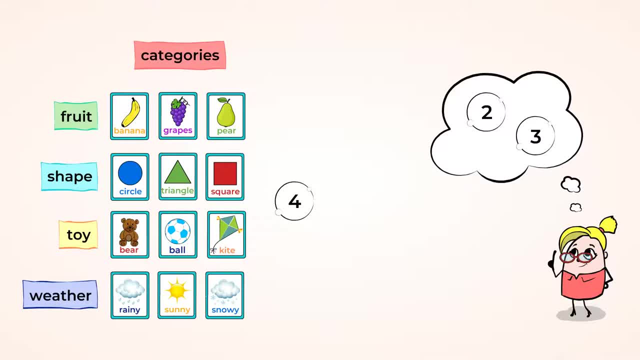 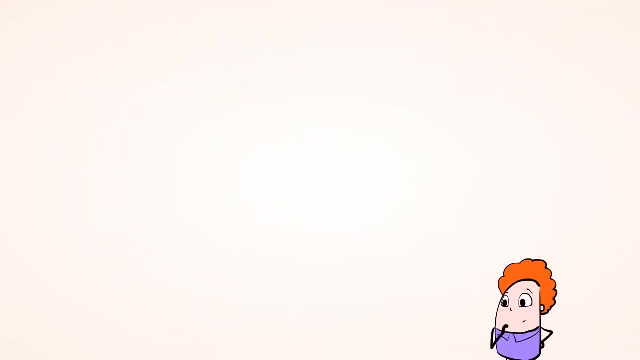 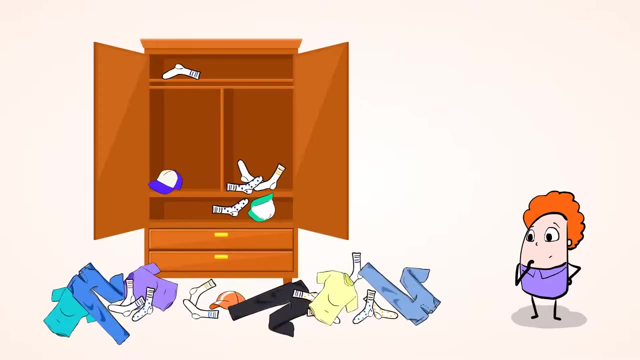 Now that all her cards are organized, Jenny can put them back in their box. Thanks so much for helping her out. Because you're so good at making categories, do you think you could help Eric organize his closet? Eric's clothes are all over the place. 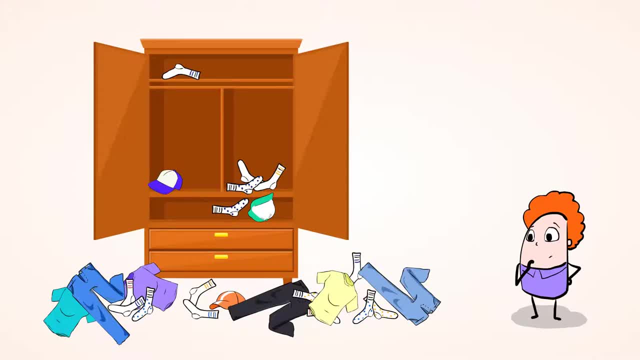 and it's really hard for him to find what he needs to get dressed in the morning. Let's help him put his clothes into categories. The first thing Eric puts on in the morning is a shirt, So let's make a shirt category. These shirts can all go in this part of the closet. 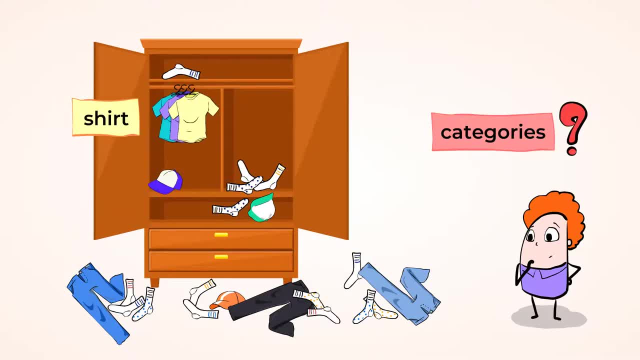 What other categories could we make? Right, a pants category. Let's put all the pants over here. His closet is looking better already. Uh-oh, there are lots of socks still lying around. Let's put them together into a sock category over here. 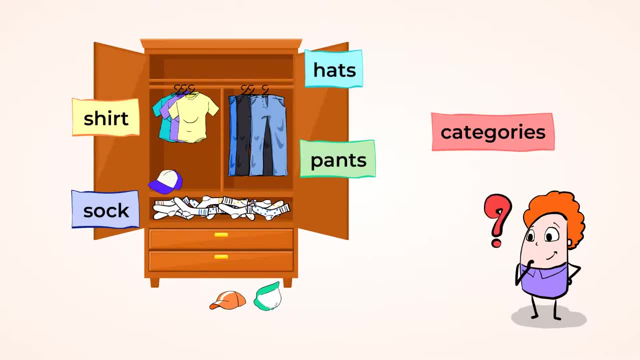 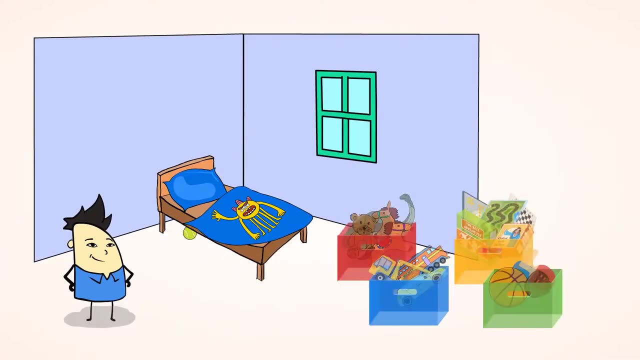 What's left, Right hats. We can put the hats together up here, And there we have it. We have a well-organized closet. Eric is so thankful for your help. Oh hey, here comes Chen. He has four toy boxes in his room. 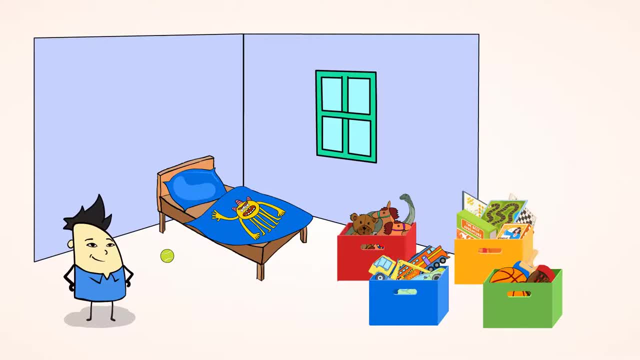 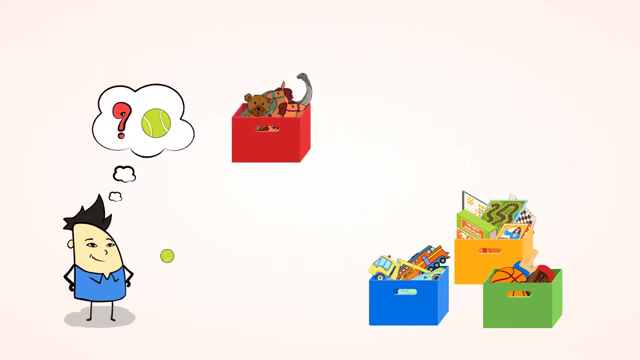 and he just found a tennis ball under his bed and wants to know which box he should put it in. Can we help him? Let's look in the first box. It has dinosaurs, teddy bears and horses. Looks like this is the animal box.